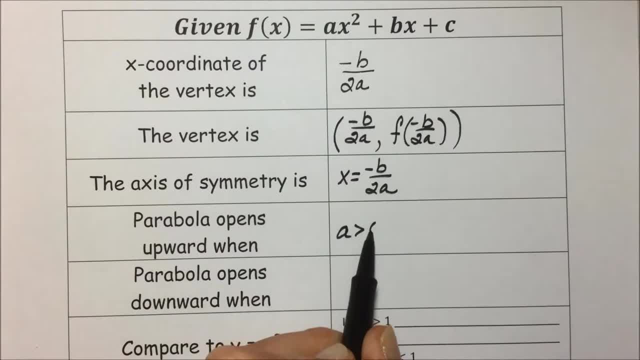 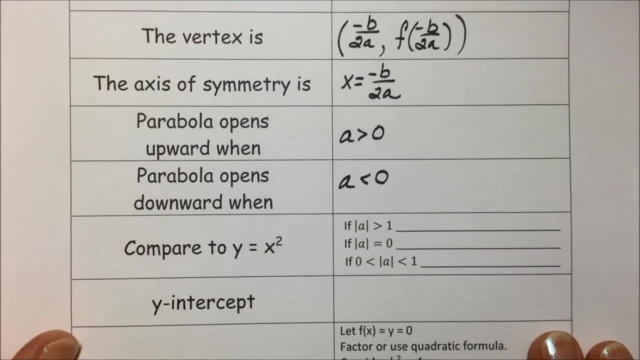 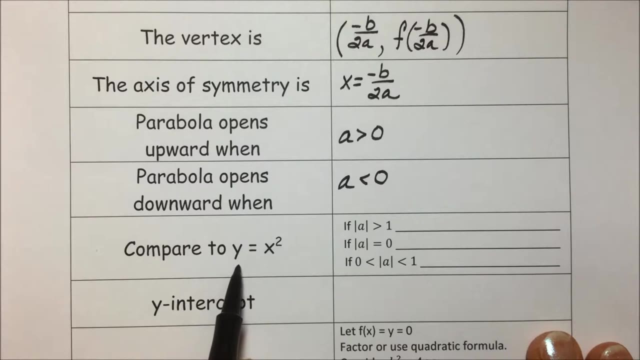 will open upward when a is positive, which means it's greater than zero. It will open downward when it is less than zero. Comparing our quadratic functions to the very basic quadratic form of this equation, if the absolute value of a is greater than one, then our parabola: 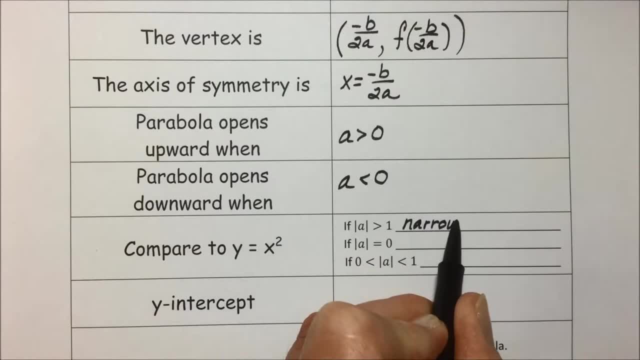 will be narrow and head towards infinity much faster. If a is equal to zero, it will be the same- Actually, this should be equal to one. And if our a, the absolute value of it, is a rational number between zero and one, then we have a squatty much wider, slower to approach. 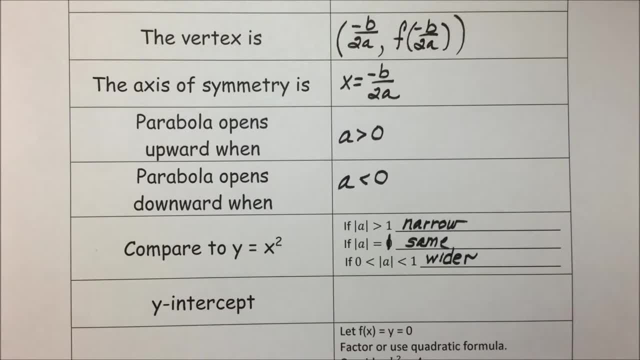 infinity than the generic y equals x squared term For a y-intercept. we let x equal zero and when we let x equal zero we have a square root of zero. So we have a square root of zero. If we let x equal zero in our equation we end up with c for our value. So the point. 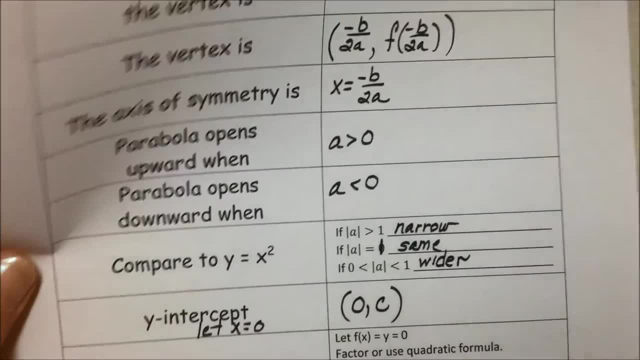 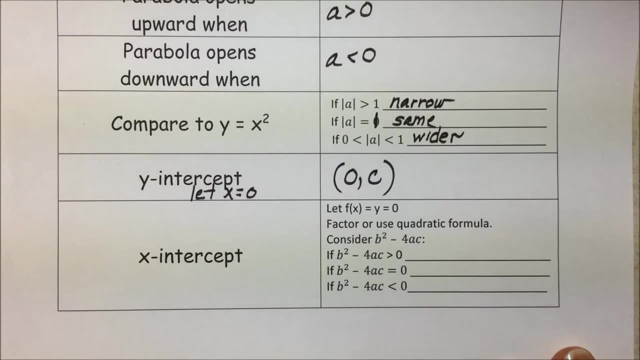 of the y-intercept is at the coordinate zero c. To determine our x-intercepts, where the parabola will cross the x-axis, it can cross in several possibilities or not at all. And so, to find the x-intercept, we let the f of x, which is actually our y, equals zero. 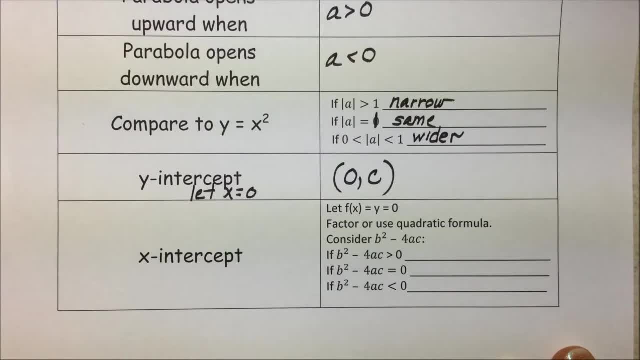 into the square root of zero. We can either factor or use the quadratic formula to find our x-intercepts, which are the roots or solutions to the equation, depending on the application of the quadratic formula or equation. But to help us along the way to find the x-intercepts, 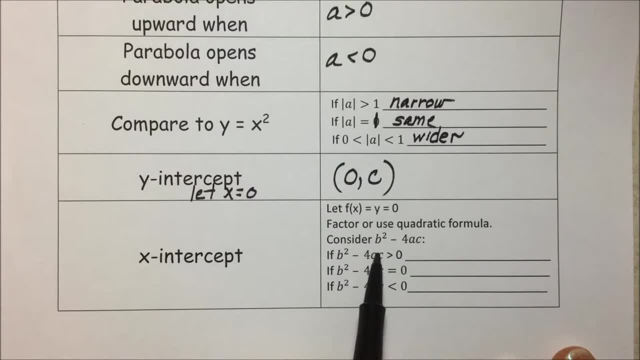 consider the discriminant, which is the radicand from the quadratic formula b squared minus. If that discriminant is greater than zero, it means that we have two real roots. It could be rational or it could be irrational. If our discriminant is equal to zero, then we have one real root. 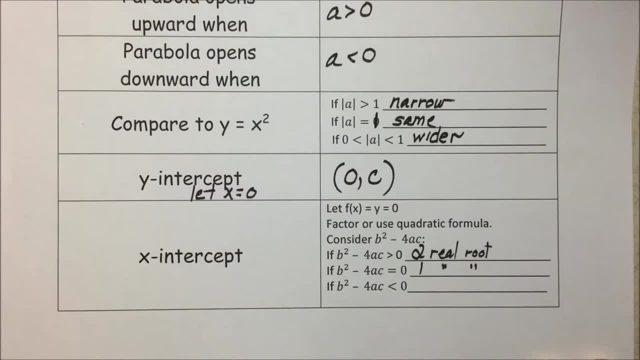 and it means we only have one intercept. If the discriminant is less than zero, we would have two imaginary conjugates. Well, we're graphing only real numbers, which means, in terms of our graph, we would have no x-intercept. 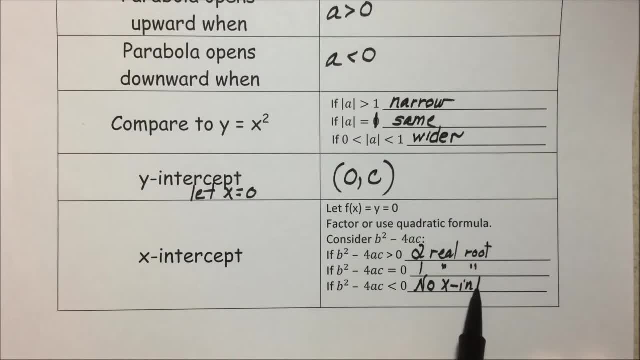 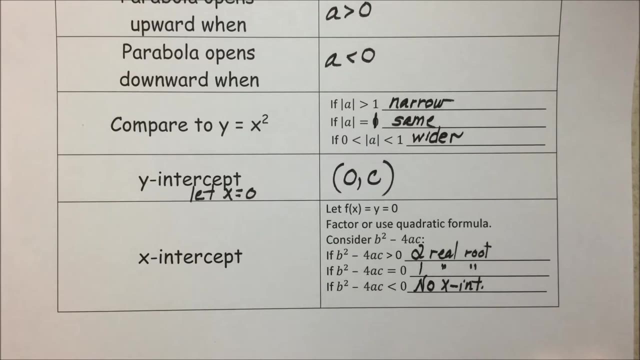 The parabola would either open above the x-axis or it would open below the x-axis with no intercept and we would have two imaginary conjugates. Okay, And in terms of solutions or roots, we would have imaginary conjugates, and again means we aren't going to graph those. 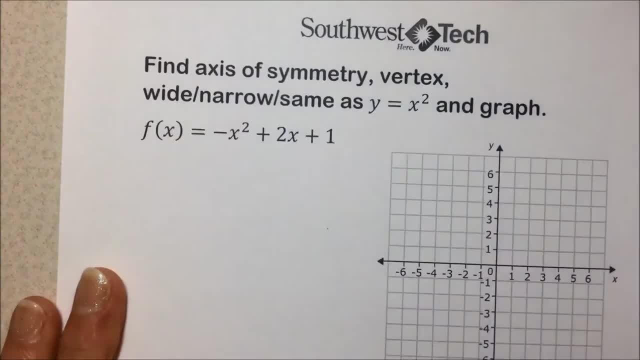 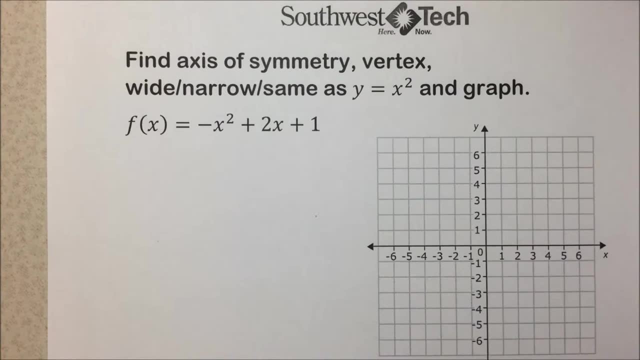 So let's put this summarized information into practice In this problem. they're asking us to find the axis of symmetry, the vertex, whether it's wide, narrow or the same as this generic y equals x squared, and then graph it. 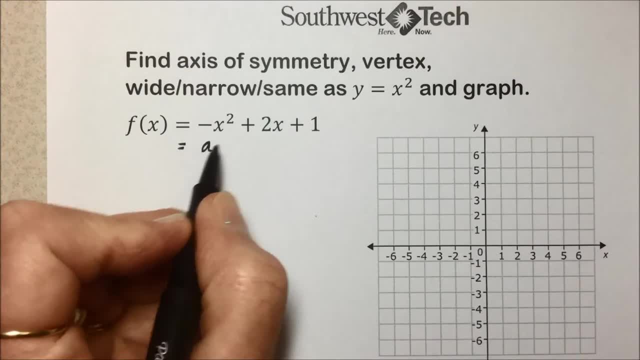 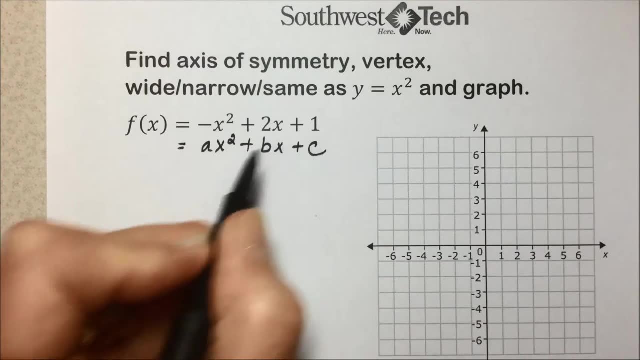 So we're going to compare this to our quadratic generic function of ax squared plus bx plus c, so that we can see that our value of a, the coefficient on our x squared term, is negative, 1,, b is 2, and c is 1.. 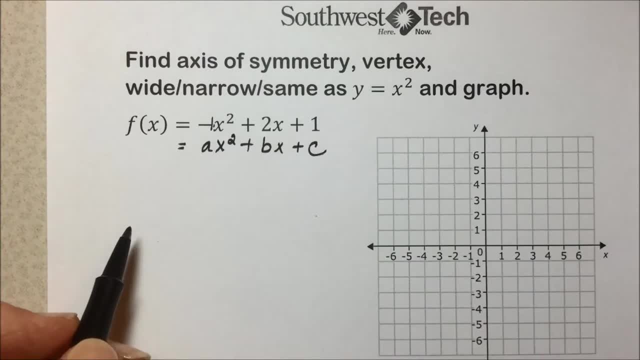 So to get our axis of symmetry and on our way to the vertex, we need to know the value of negative b over 2a. So it's the opposite of b. so it'll be the opposite of a positive 2, which is negative 2,. 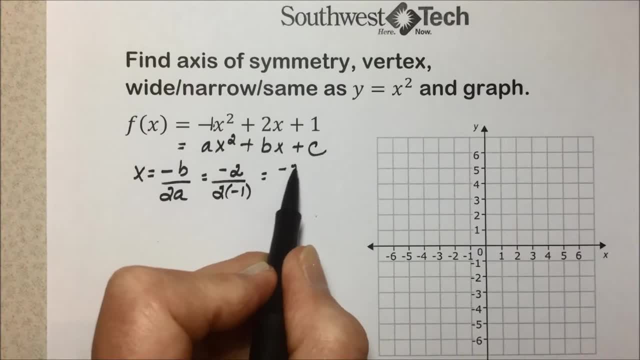 over 2 times a, which is negative 1. This will give us a negative 2 over negative 2, which results in: 1.. Plugging that x into the function will give us the associated y value so that we can have the coordinates of the vertex. 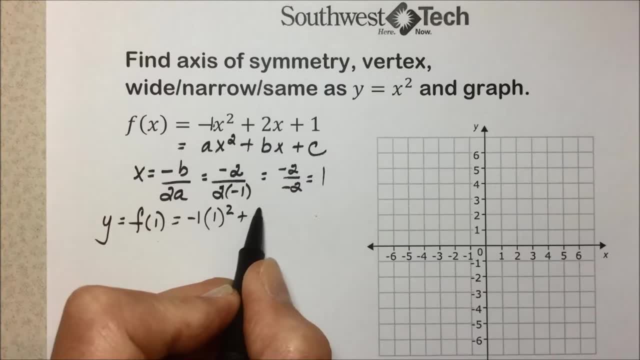 So replacing x with a, y With a 1 and simplifying 1 squared is 1 times negative. 1 is negative 1.. Multiply is 2 plus 1.. Negative: 1 plus 2 is 1.. 1 plus 1 is 2.. 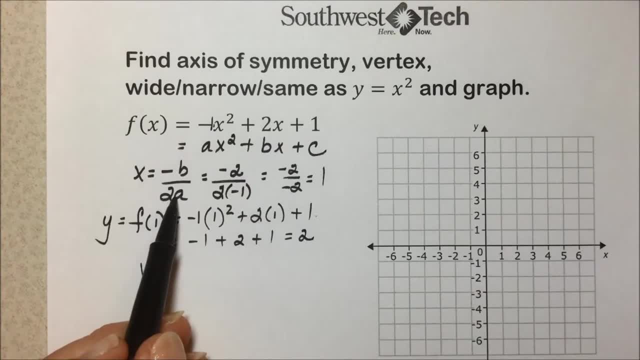 So to identify the vertex which is negative, b over 2a. for the x coordinate we found a: 1. Plugging that value into the function, we have the associated 2.. So the vertex of this quadratic function is 1, 2.. 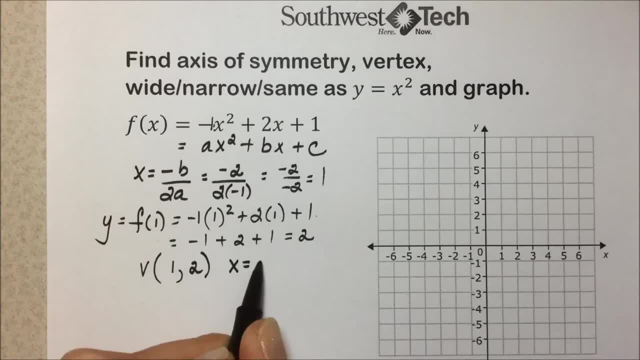 The axis of symmetry is x equal the x value of our vertex. It always runs through the vertex. So there's our equation for the axis of symmetry To determine the shape of the parabola we need to look at a. A is equal to negative 1.. 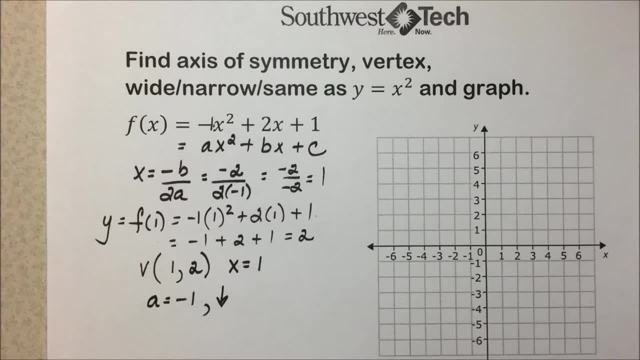 Since this is negative, the parabola is going to open downward. That helps us with getting an estimate for the graph. But to answer the question, if we have the absolute value of a being greater than 1, the graph will be narrow. 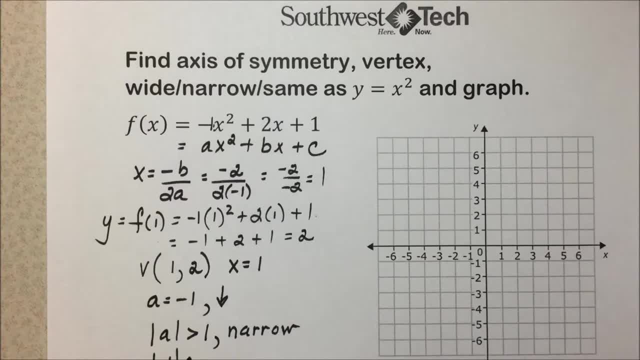 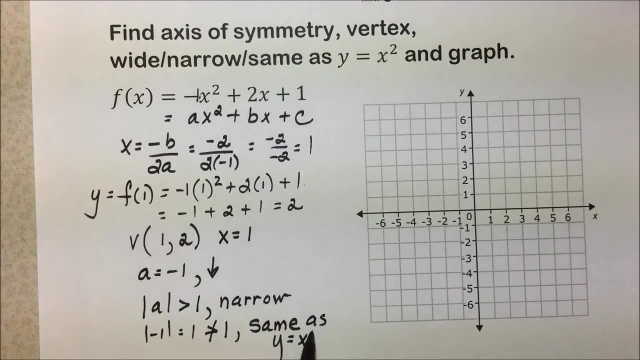 Well, when we plug in a negative 1,, the absolute value of negative 1 is 1.. That is not greater than 1.. It's equal to 1, which means it's going to be the same shape as the y equals x squared form. 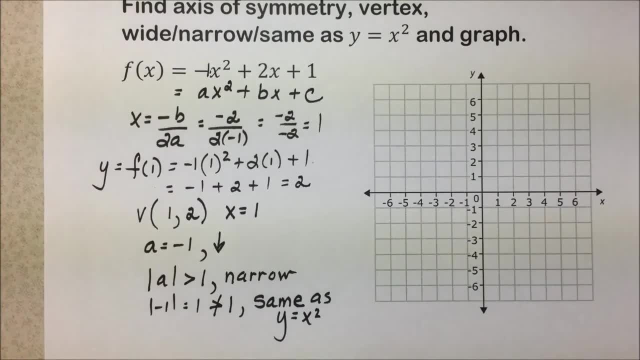 One other point just to graph. this is needed because we can use the reflexive property about the axis of symmetry. A very easy point to find is the y-intercept, which generically is the coordinate 0, c, And on this quadratic function, c was 1.. 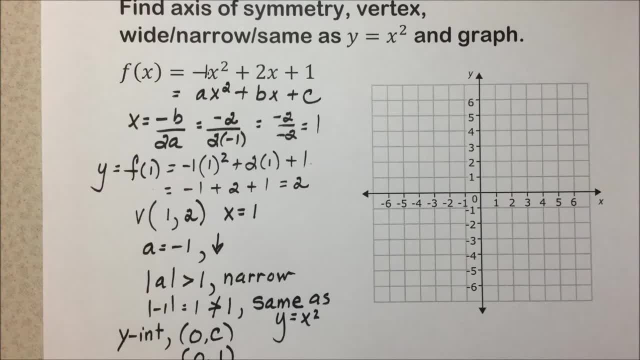 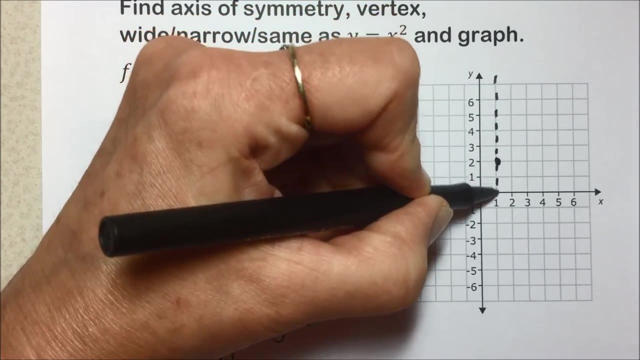 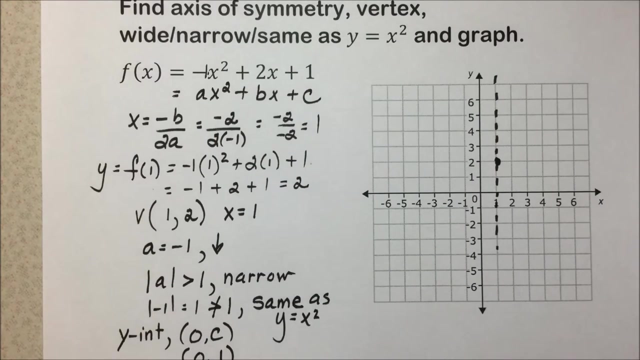 So we have the point. So, taking these components, let's make a graph for this quadratic function. We have a vertex at The axis of symmetry is running through the vertex. It's at the line x equals 1, a vertical line. 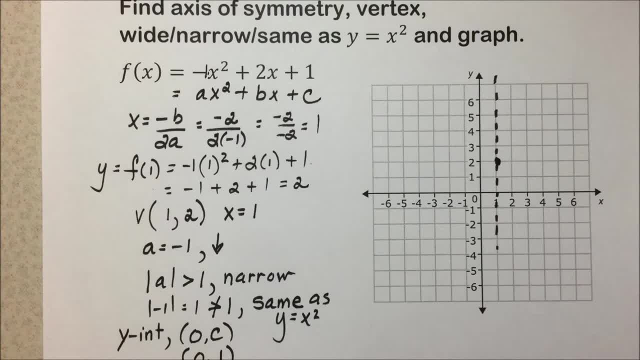 We also know that we have a y-intercept of, Because we are 1 away from our axis of symmetry. we can, through reflexive, find another point And we could verify that if we let x equal 2, plug it in. 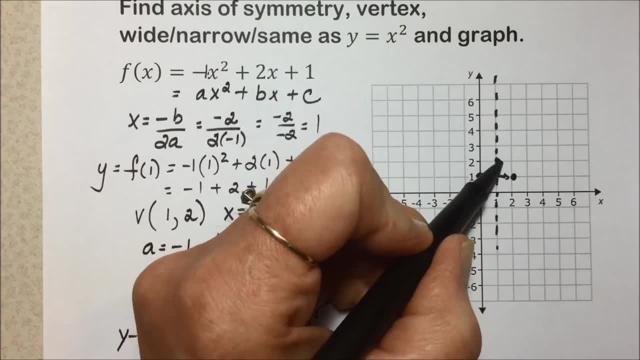 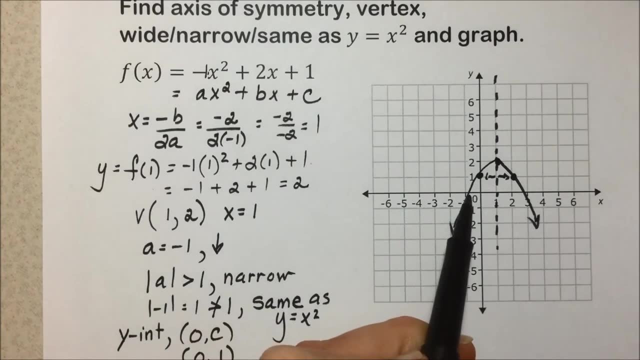 we should find that it has a value of 1. Connecting these with a smooth line. we have our parabola Now where they're intersecting on the x-axis, for the x-intercepts aren't exact here, but the problem is not asking us for that just yet. 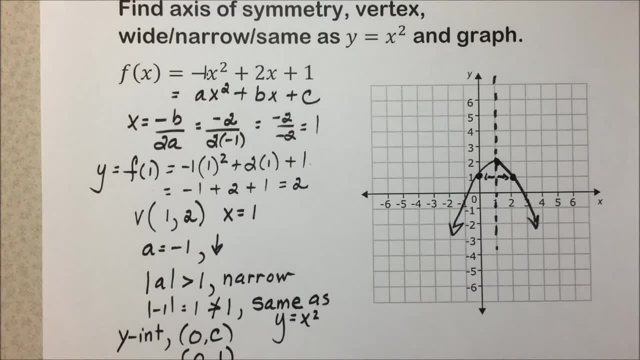 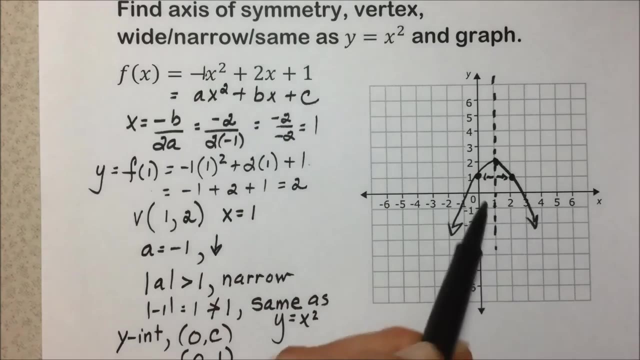 We'll take a look at another problem In the future to have exact values. But our parabola is opening downward as we expected. We have identified our vertex at the point. Our axis is symmetry. We have one point that we reflected to get a second point for a general shape. 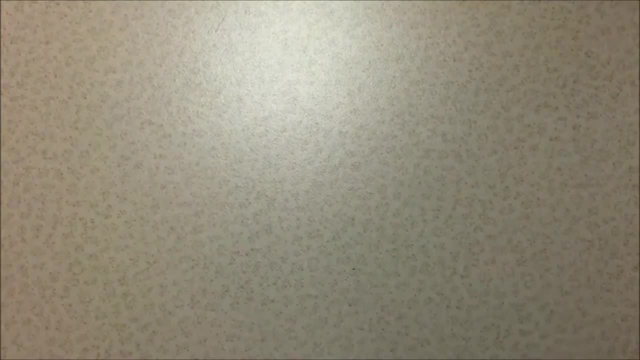 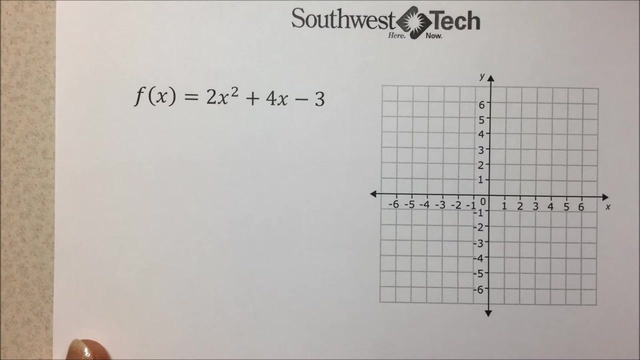 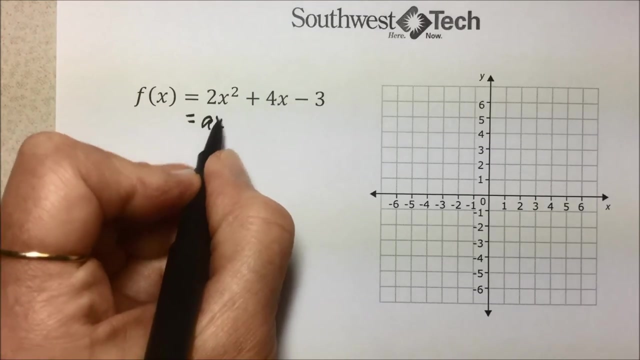 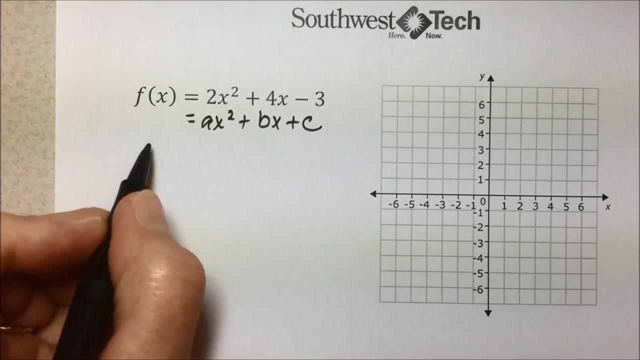 for this problem. Let's look at another problem that's asking the same information: Find the axis of symmetry vertex and the shape of it, as well as graphing it. So, comparing this ax squared plus bx plus c, we have a of 2, b of 4, c of negative 3.. 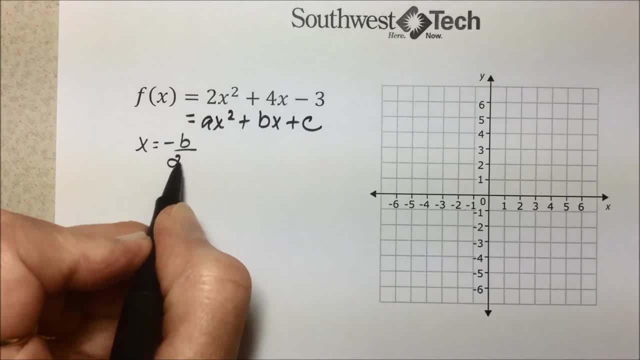 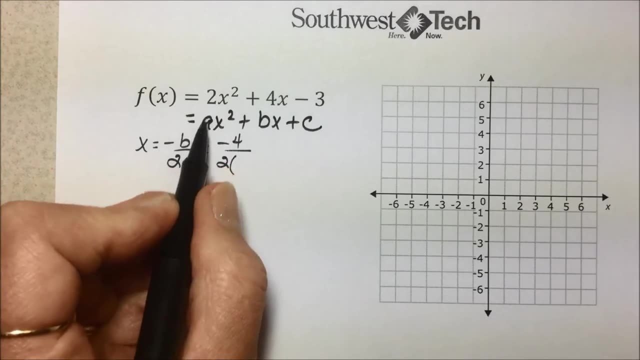 We can find the x-coordinate of the vertex by taking the opposite of b, which is going to be a negative 4, over 2 times a, which is a 2. We end up with a negative 4 over 4,, which is negative 1.. 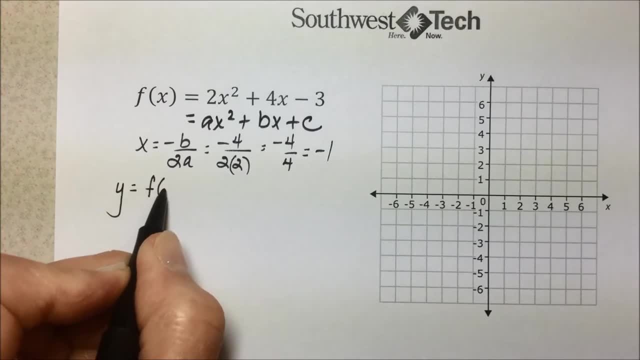 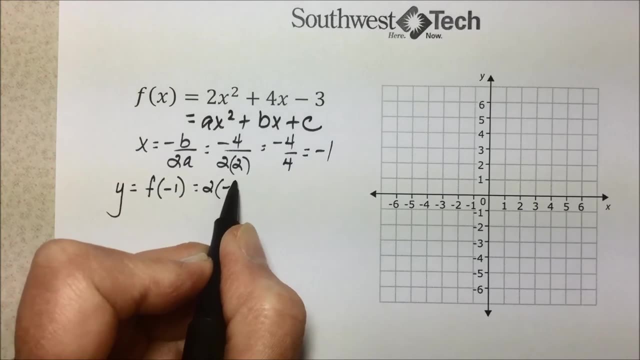 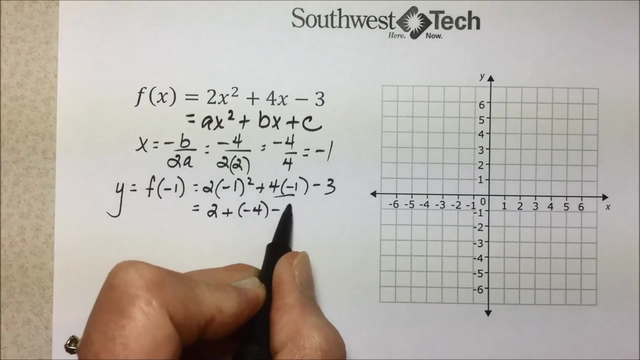 To find the corresponding y, we will plug or replace x with negative 1 into our quadratic function Powers first, negative 1 squared is 1, times 2 is 2.. Multiplying next we get a negative 4, simplifying 2 plus negative 4 is negative 2,. 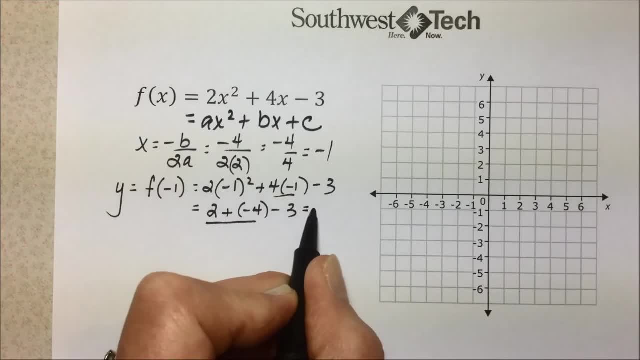 negative 2 minus 3 or plus a negative 3 is negative 5.. So our vertex, which is negative b over 2a for our x f of that value, gave us a negative 5.. The axis of symmetry is x equal, the x value.